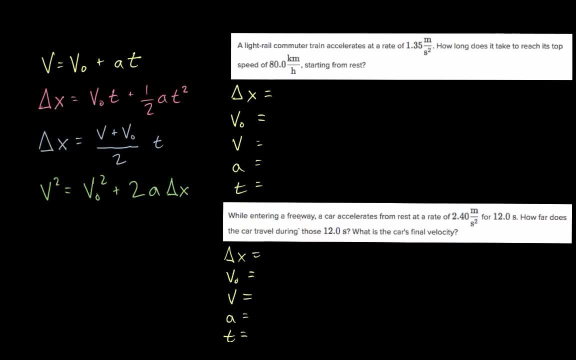 is doing when you use it. but once you understand that the calculator is a really valuable tool, And that's what these equations are like- They're tools that we can use when we understand where they come from. So with that out of the way, let's dive into our example here. 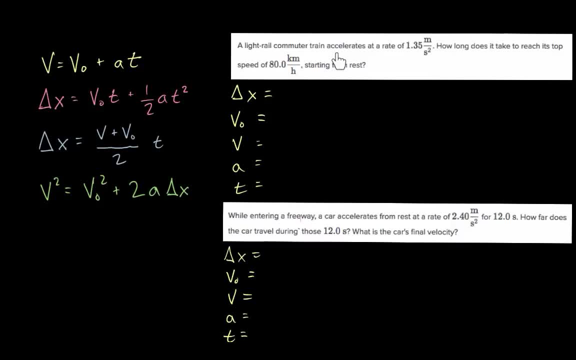 So the question says: A light rail commuter train accelerates at a rate of 1.35 meters per second squared. How long does it take to reach its top speed of 80 kilometers per hour, starting from rest? All right, so let's unpack this and see what it's saying. 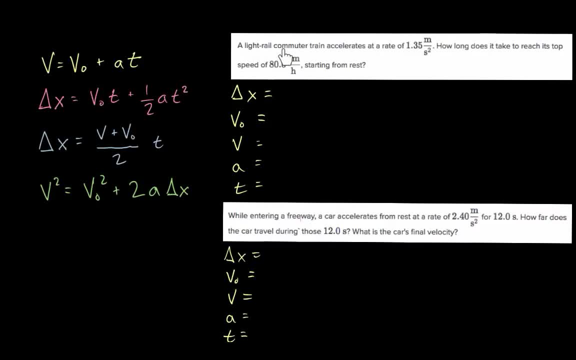 So let's just start at the beginning. A light rail commuter train accelerates at a rate of 1.35 meters per second squared, So that's pretty direct. It's just telling us what the acceleration is, So let's write that down. 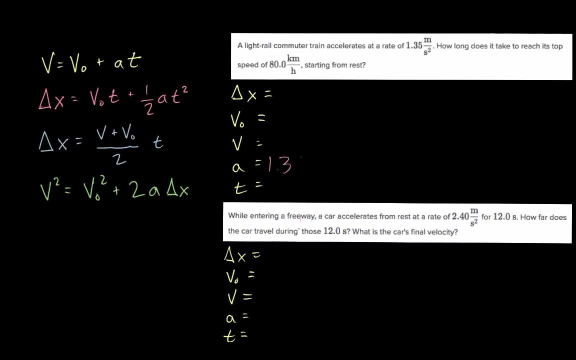 The acceleration is 1.35 meters per second, squared. All right, there's one thing Okay, so let's keep going. How long does it take to reach its top speed of 80 kilometers per hour, starting from rest? So that one's a little bit more complicated. 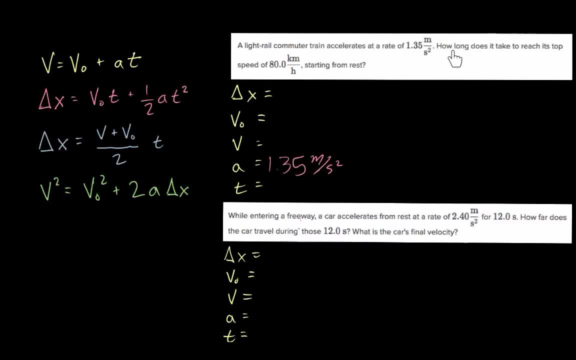 There's more going on in here, But if we just start at the beginning and say, how long does it take? right, That by itself is a question. There's some more stuff afterward, but that by itself is just asking about the time. 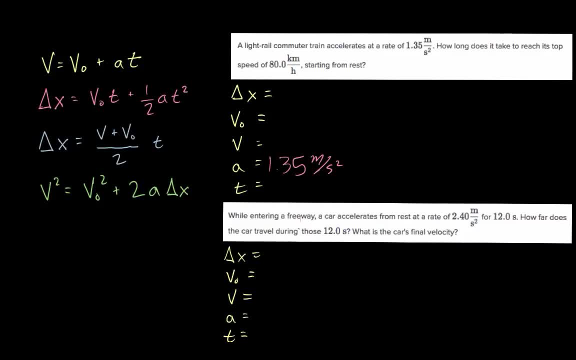 How long does it take? All right. so let's note that by circling this time here, We don't know what it is yet. but this is our question. We're being asked It's about the time, All right. so if we keep going here, we get all right. how long does it take to reach its top speed of 80 kilometers per hour? 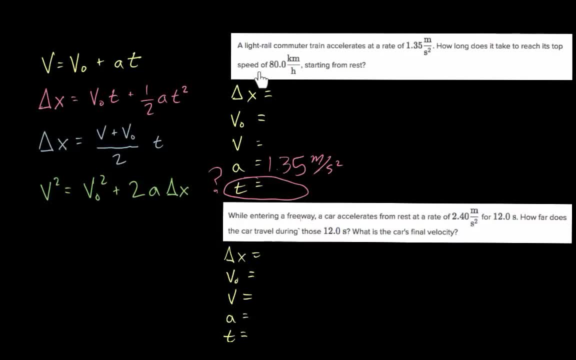 So that's saying its top speed is 80 kilometers per hour. When it's done speeding up, it'll be going at 80 kilometers per hour. So that's the final velocity, or just our velocity at the time here. So that's 80 kilometers per hour. 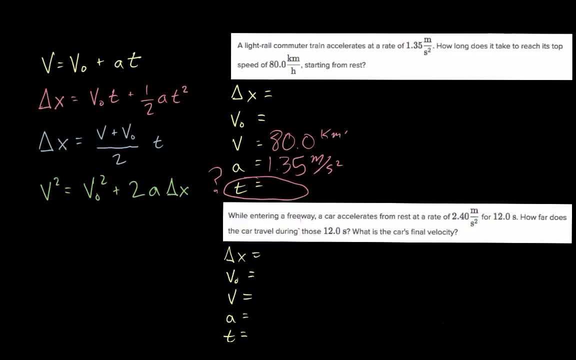 80.0 kilometers per hour, And sometimes you'll see this right here written as V, sub F, to really explicitly say it's the final velocity. So the notation might vary in your physics class, But so whatever notation you use, that's fine. 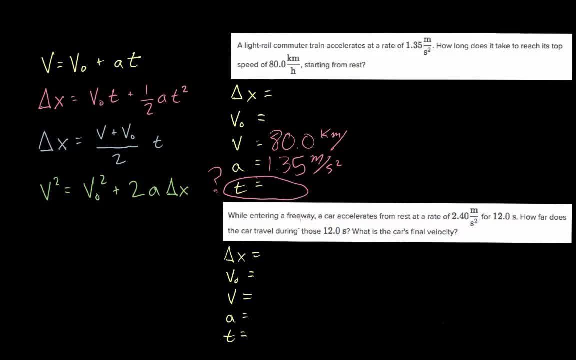 But make sure to ask yourself: what is this symbol really talking about? So, anyway, 80 kilometers per hour, Per hour, Okay, And so we have that. And then, if we keep going, it says starting from rest. So that's saying that at the beginning, when it starts, it's at rest, which means it has zero for its initial velocity. 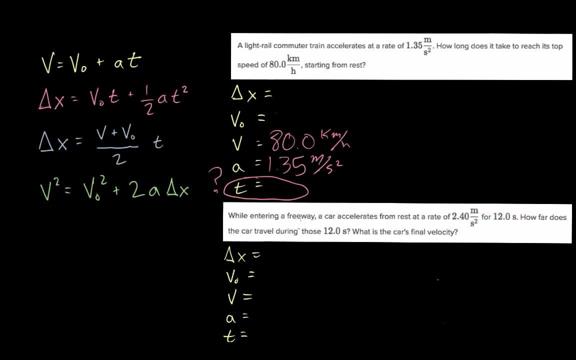 It's just sitting there, So let's fill that in. That's zero meters per second. Okay, So we have analyzed this question and we see that actually the change in distance didn't appear anywhere in this question. It's just these four values right here. 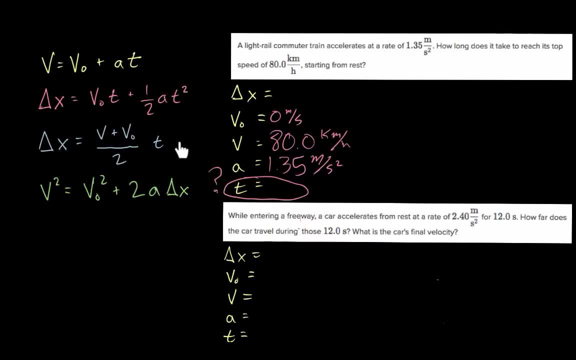 So let's see if we can look at these equations and identify one that has all of these things and doesn't have delta x, Since we don't know delta x and we're not looking for it either. So we see these two have delta x here. 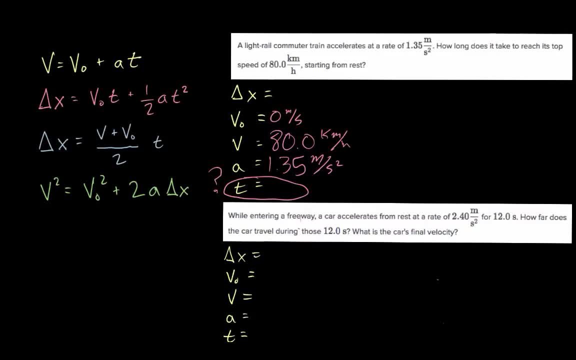 And so we can rule those out. And this one also has a delta x, so we can rule that out. So that leaves this one. Let's see. It has velocity, the final velocity here. It has the initial velocity here. It has acceleration here. 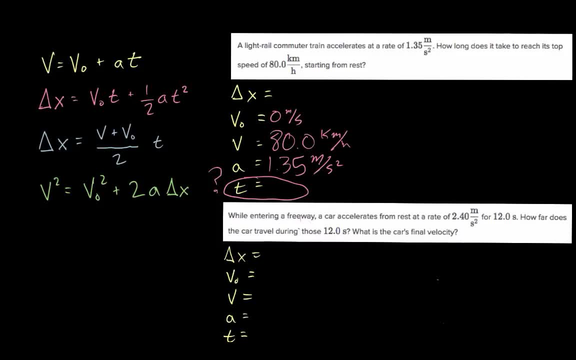 And then it also has time, which is what we're looking for. So we can use this. We've figured out that for this question right here, we can just use that top equation, All right. And then to continue this, we would plug in numbers and then solve for t and see what that time indeed is. 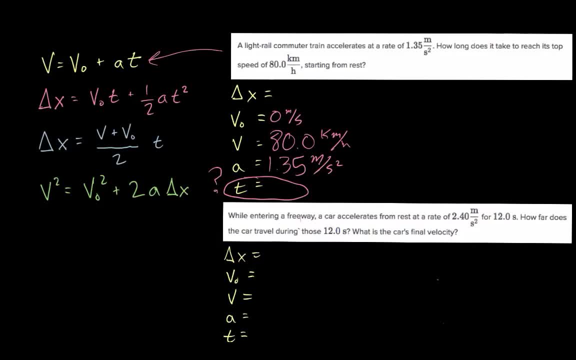 So for this Video, we're not going to actually go through that, We're just going to go through another example of setting things up. So let's go down to this question right here. While entering a freeway, a car accelerates from rest at a rate of 2.40 meters per second, squared for 12.0 seconds. 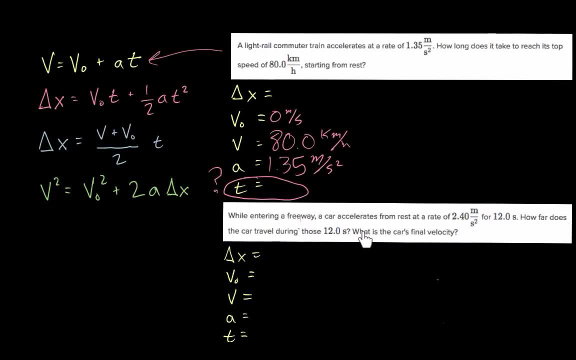 How far does the car travel during those 12 seconds And what is the car's final velocity? So this one actually asks two questions. So let's just let's just focus On on the first one to begin with, And also let's see what we know. 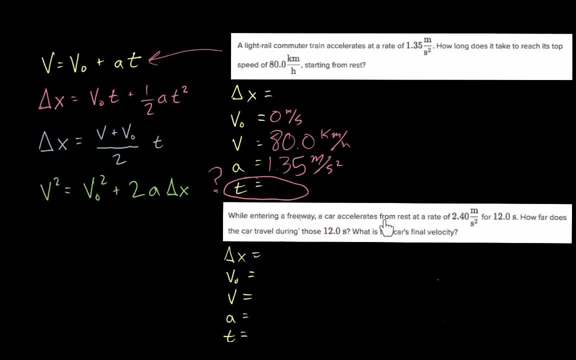 So, while entering a freeway, a car accelerates from rest at a rate of 2.40 meters per second for 12 seconds. So there's a lot of information here in this first sentence. So let's, let's see. It says accelerates from rest, right here. 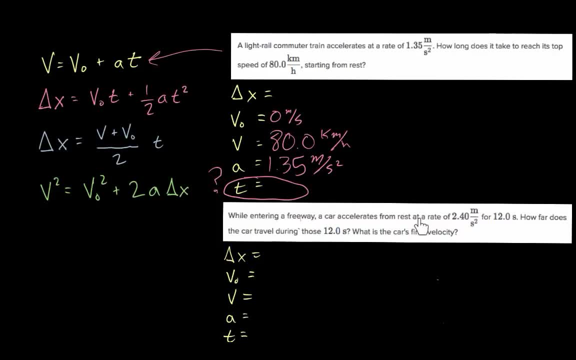 Accelerates from rest. That tells us that the initial velocity is zero, right from rest. It wasn't. it wasn't moving initially, It was At rest. So let's write that down. This also, just like the previous example had a had an initial velocity of zero meters per second. 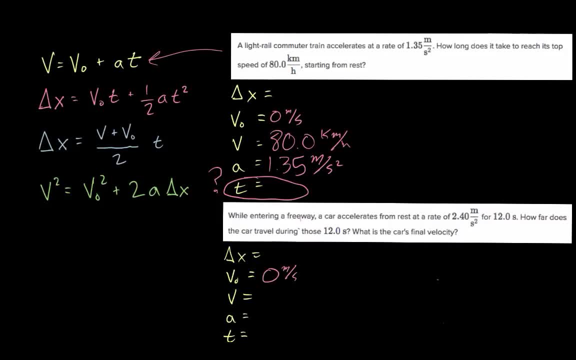 That's not always the case, but it happens that in these two examples it was: Let's keep going. So it accelerates from rest at a rate of 2.40 meters per second squared. So that's, that's telling us what the acceleration is. 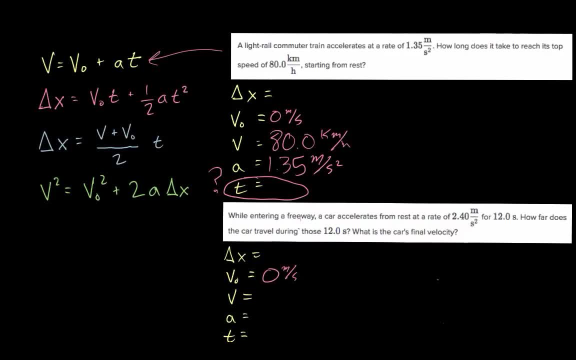 2.40 meters per second squared. Let's write that down: 2.40 meters per second squared. meters per second squared. and in all of these problems it's important to think about whether something is moving in the positive direction or in the negative direction, or if it's accelerating in the positive direction or the negative direction. it actually looks like for these examples we've chosen: everything is, is is moving in the positive direction and accelerating in that same direction. 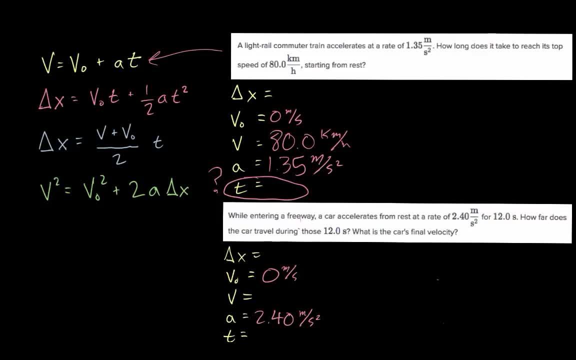 So we won't have any negative signs pop up. but it is important to think about that when you're doing these kinds of things, just just in case something is negative And that does that does affect your answer and what's going on. But anyway, so so it's accelerating forward, everything's going in the same direction. 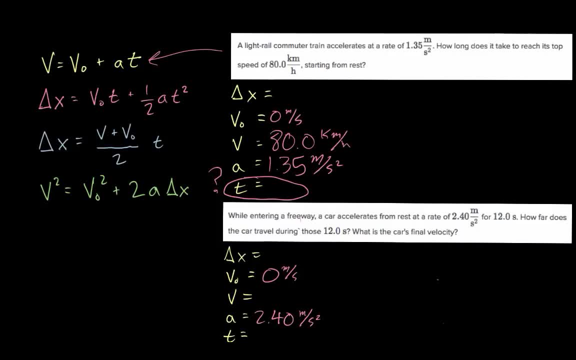 So we're thinking of forward as the positive direction and they're accelerating that. this, this car is accelerating at 2.4 meters per second, squared, All right. and it says also that it's doing that for 12.0 seconds, so we can write that down as well. 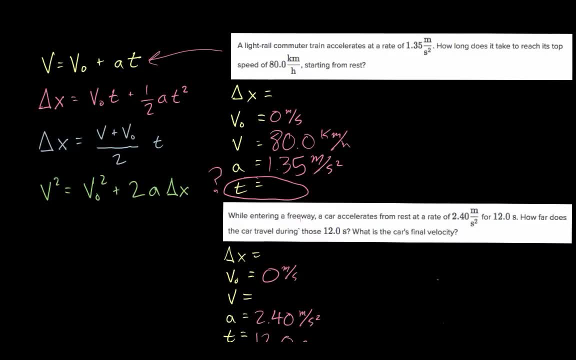 12.0.. 12.0 seconds. All right, so we know. we know three things here, and you'll find that in problems like this, that's the magic number. Once you have three of these, you can- you can- find out the other pieces using these equations. 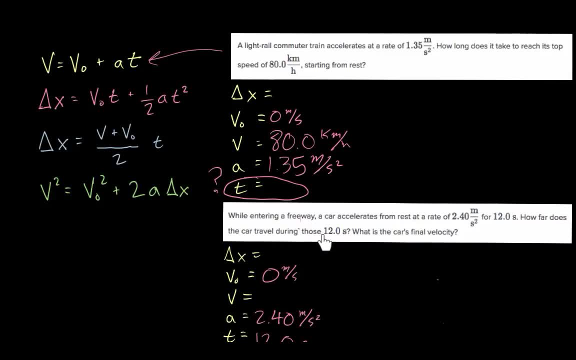 Anyway. so the first question says: how far does the car travel during those 12.0 seconds? Well, it's asking how far So that's going? It's going to be the delta X here, this change in position. How far does it travel during those 12 seconds? 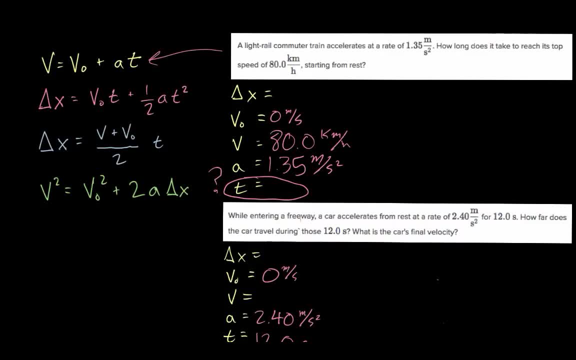 It's going to be this, this value, right here. So this is our question, Circle it here. So now notice, we don't have this. So we can look for an equation that doesn't have this, this final velocity value, in it, And then that will be an equation that will hopefully have these other four. 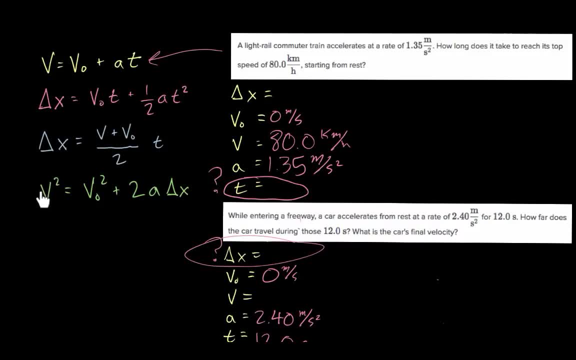 But we'll have to check that. So this one It has that final velocity in it, so we can rule that out. I see this one also has the final velocity. This one doesn't have the final velocity, So let's look at that. 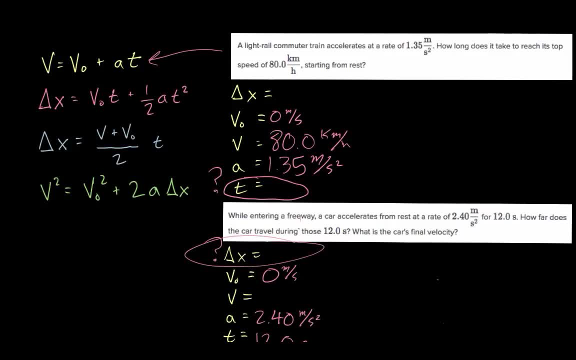 Does it have? So it has the position, the change in position. That's what we're looking for. It has it right there. The- or sorry, the initial velocity is right here, So we have that as well, Let's see. 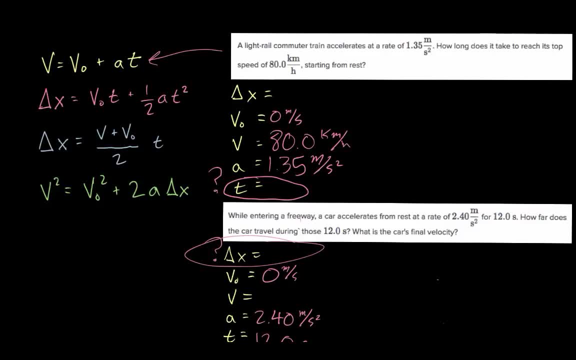 It has time in it and we have time, So we will be able to plug that in. And then, finally, it also has acceleration. So we have that, So we have that. So it has everything we need. It has the thing we're looking for. 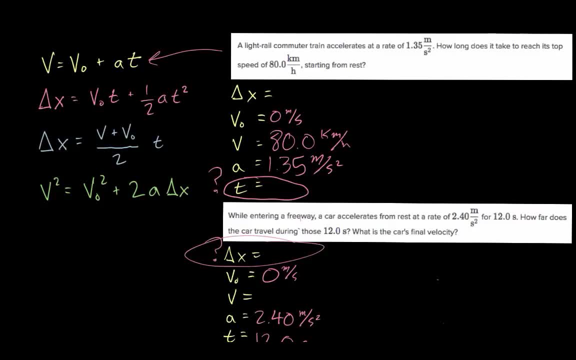 And and it and it doesn't include anything that we, that we just don't know, that we're not even looking for. So we found that for this problem right here, This second equation here is going to be the one that is most useful for asking, for answering the question: how far does the car travel during those 12 seconds? 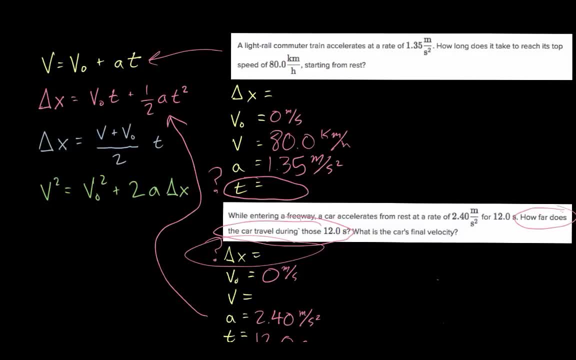 So that's, that's for That question. But this, this block here actually has a second question. Maybe I'll switch to green, Let's. let's look at this question. What is the car's final velocity? So All right. So that means we're looking for this now. 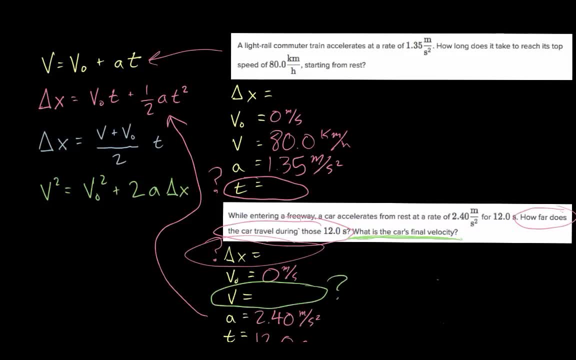 Right here. What's this? Well, we've already identified these, these different pieces that we know, And if we did the first part of the problem, we would actually have a value for for Delta X here. But assuming we didn't, we didn't find that yet. 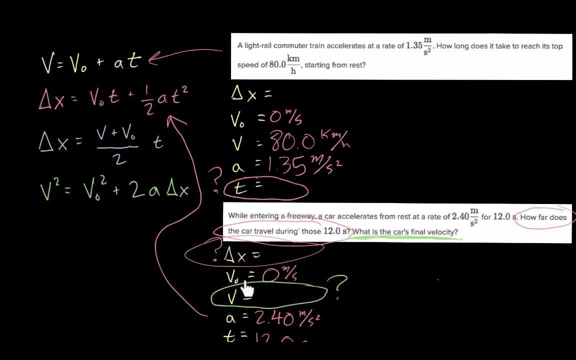 We could look at this and say what's the car's final velocity. I want to look for something that has V in it and and has these other three things that I know, And if you look and you check through here, let's see what is it. 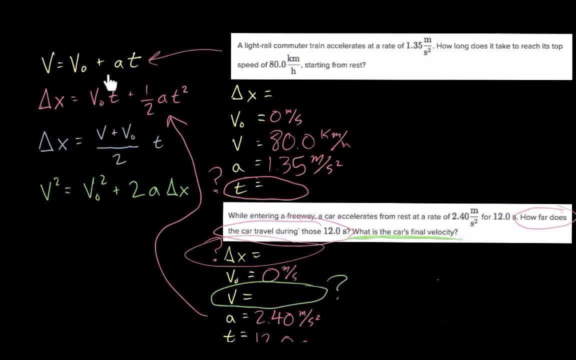 So, yeah, it would actually end up being this one again. This is that, that equation that doesn't have the change in position in it, And so just using the green color, I'll I'll underline this here to say that This equation is useful for it, for this question. 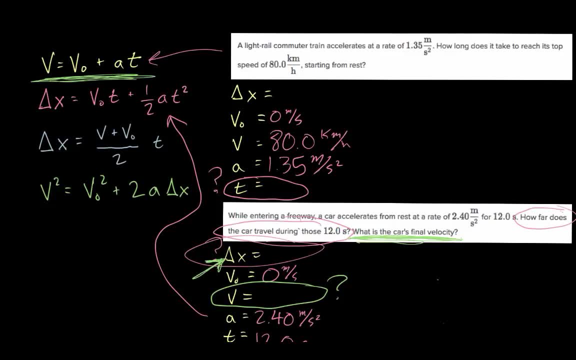 And actually now that now that we have this value, we could have used really any of them that had had our V in it. So our options open up once we know more than three different things. But anyway, hopefully going through a couple of these examples that will be helpful for you when you run into your own questions and have to think through: OK, what do I have? 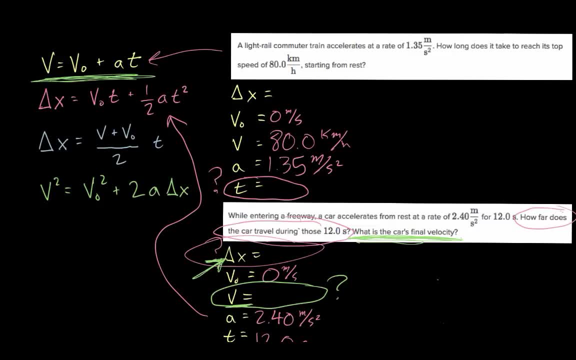 What am I looking for And which equation? Which equation will help me move forward and solve this question? 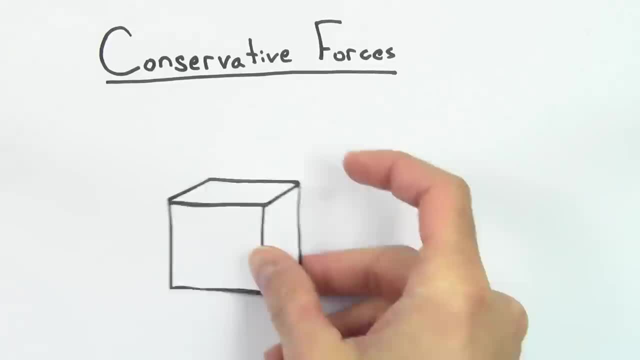 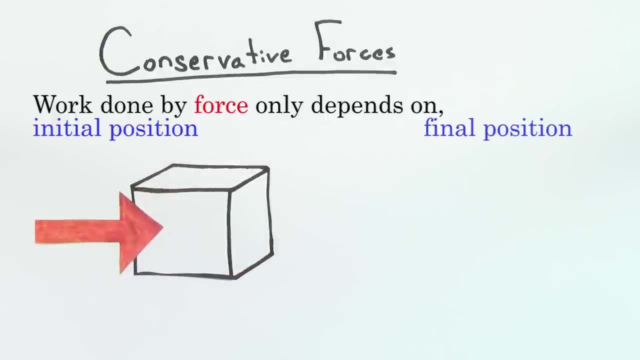 What's a conservative force? Conservative forces are any force wherein the work done by that force on an object only depends on the initial and final positions of the object. In other words, the work done by a conservative force on a mass does not depend on the path taken by that mass. 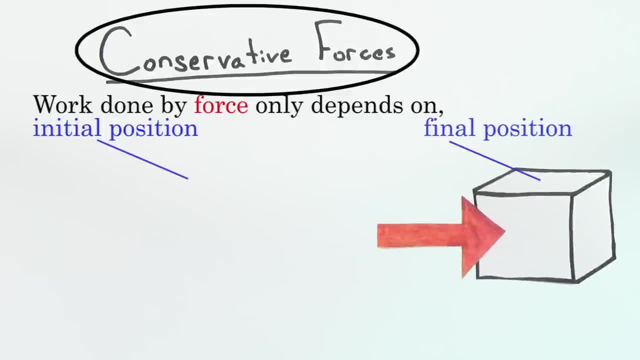 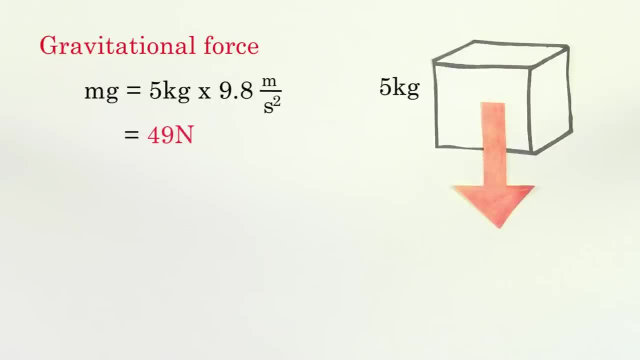 If the work done by a force follows this rule, then we call it a conservative force. For instance, the gravitational force on a 5 kilogram mass is 49 newtons If the mass moves downwards by an amount of 6 meters. 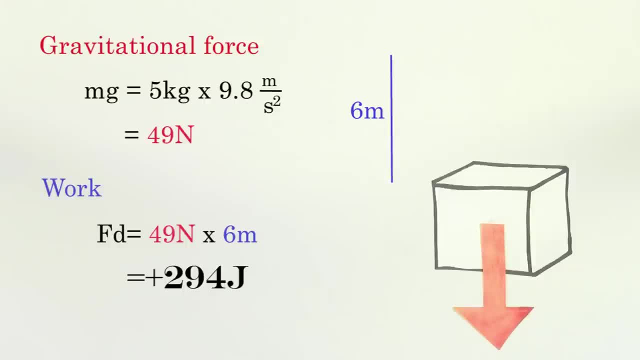 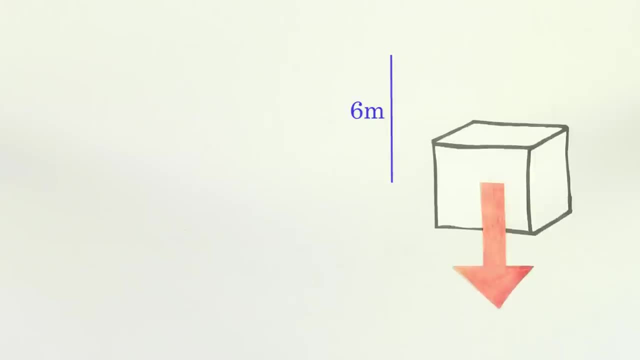 the work done by gravity is going to be 294 joules. Now let's start over. Say the mass again moves down 6 meters, but then it moves up 6 meters, then down again 6 meters. The work done by gravity for the first downwards trip was 294 joules.